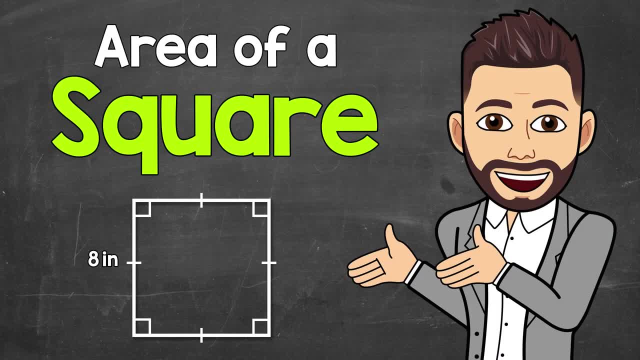 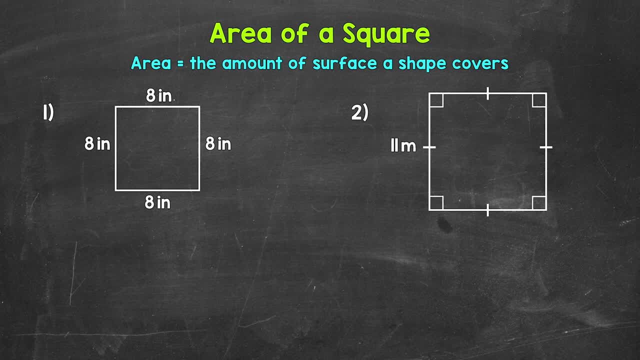 Welcome to Math with Mr J. In this video I'm going to cover how to find the area of a square. Now remember, area is the amount of surface a shape covers. Let's jump into our examples, starting with number one, where we need to find the area of that square. 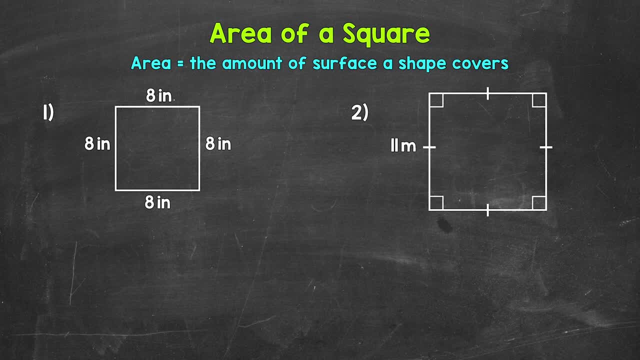 Now for squares. we can find the area by squaring a side length. So we can use the formula: area equals a side length squared And for this square each side is eight inches. So let's plug in eight inches here for our side length. So eight squared. 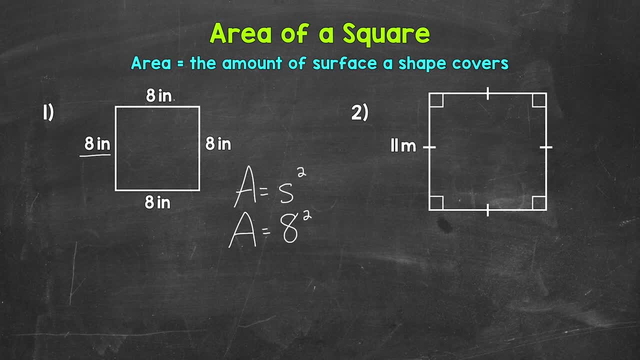 Eight squared means eight times eight, which gives us an area of 64 square inches. So eight squared equals six, which gives us an area of four inches. Let's move on to number two, where we have a square with sides that are 11 meters. 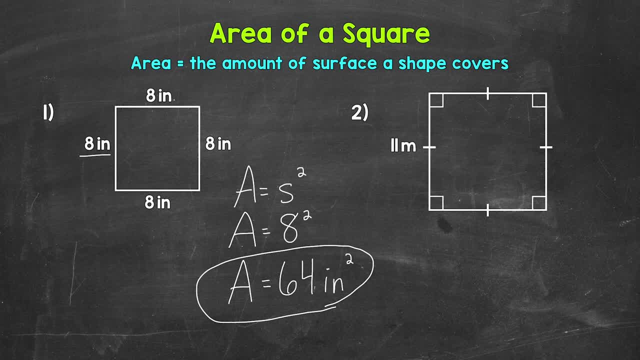 And you'll notice that we only have one side labeled. That's because this is a square and we know all of the sides are going to be the same. They're all going to be 11 meters. The tick marks on each side of this square show us that they are all the same. We have 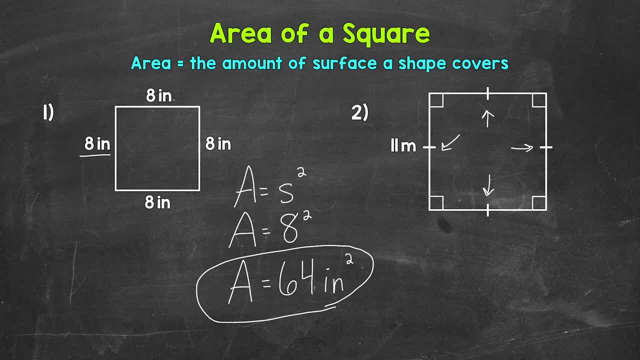 mark on each side and that indicates that, again, all of the sides are the same. Then we have the 90 degree angles marked as well. I wanted to include these symbols in case you come across them. That way you'll know what they mean As. 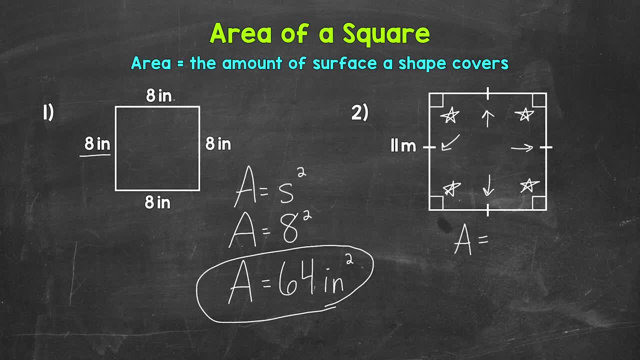 far as area, let's use the formula. area equals a side length squared, and each side is 11 meters. So let's plug in 11 meters for the side length. 11 squared that means 11 times 11. that gives us an area of 121 square meters. 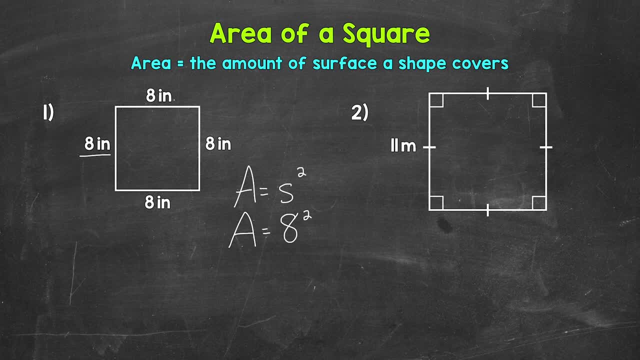 Eight squared means eight times eight, which gives us an area of 64 square inches. Anyway, let's see how we do this. So I'm going to put together this area here with an basic formula, and each side is larger than the other, So I'll close out the formula only with this formula. 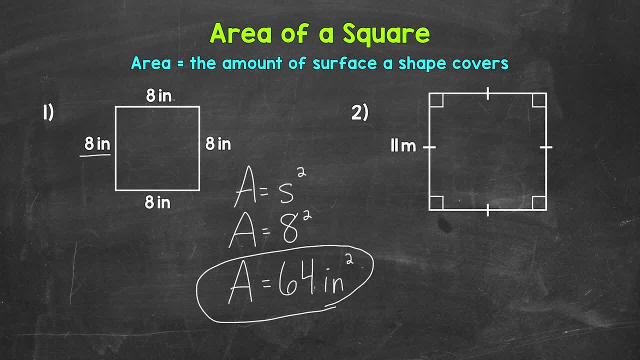 So this weird supposed square over here is nine. Alright, this one has a bigger square than the other. Let's move on to number two, where we have a square with sides that are eleven meters, And you'll notice that we only have one side labeled. That's because this is a square and we know all the sides are going to be the same. They're all going to be eleven m. The tick marks on 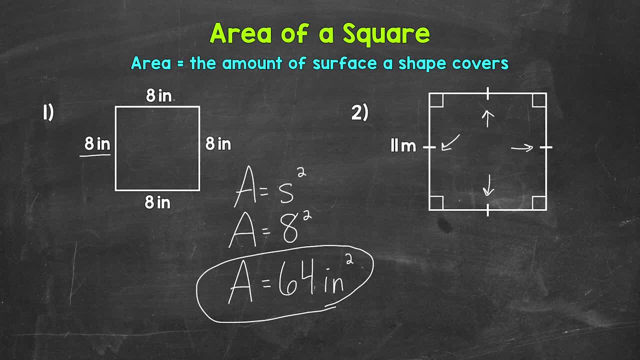 tick mark on each side, and that indicates that, again, all of the sides are the same. Then we have the 90 degree angles marked as well. I wanted to include these symbols in case you come across them. that way you'll know what they mean. As far as area, let's use the formula: area equals a side. 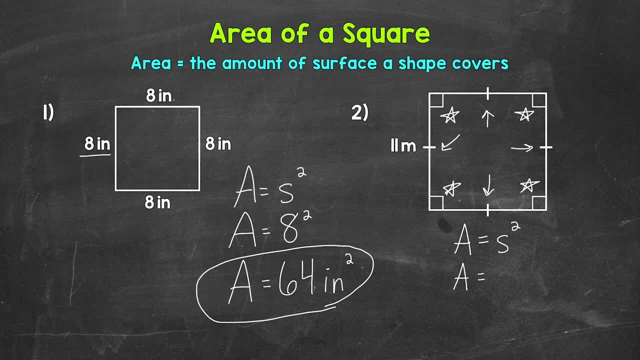 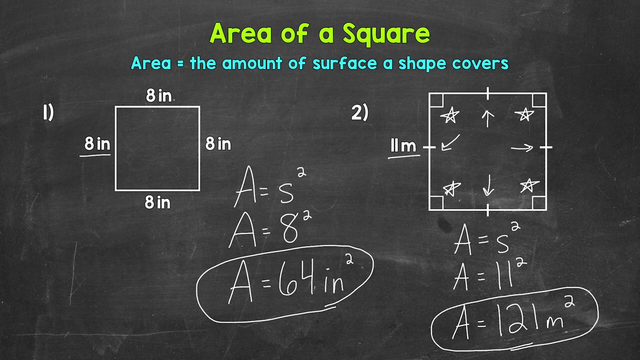 length squared, and each side is 11 meters. So let's plug in 11 meters for the side length. So 11 squared that means 11 times 11. that gives us an area of 121 square meters. So there you have it. There's how to find the area of a square. Just remember: area is the amount. 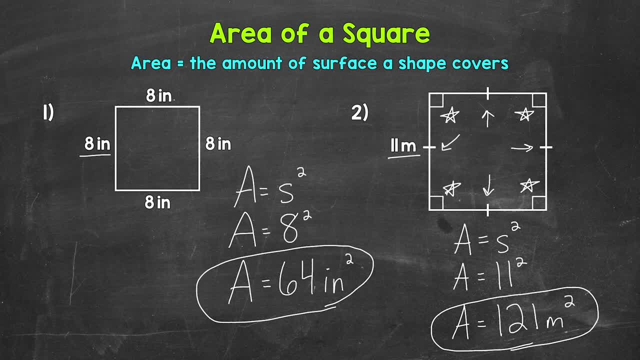 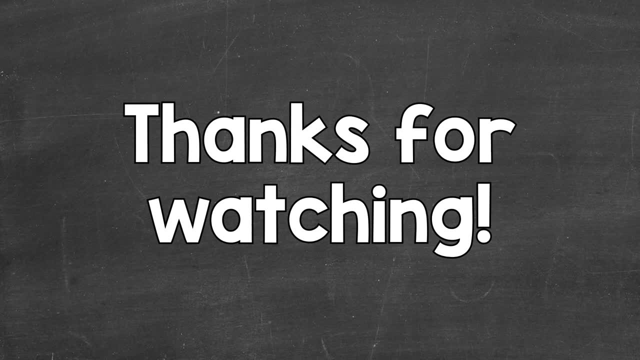 of square meters, So let's plug in 11 meters for the side length. So 11 squared that means 11 times of surface. a shape covers And for squares we can square a side length in order to find area. I hope that helped. Thanks so much for watching. Until next time, Peace.